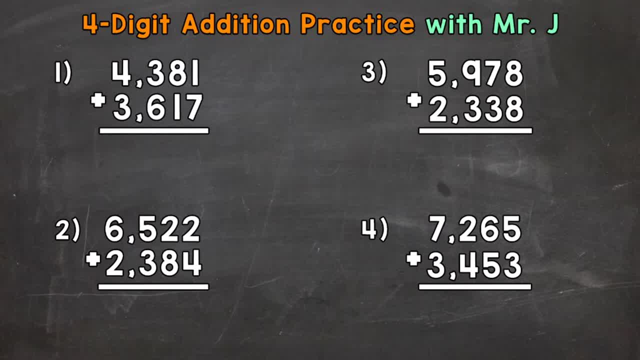 I do want to mention that some of these problems do involve regrouping. This is also called carrying. So to regroup or to carry, they mean the same thing. I'm going to use the word regrouping throughout this video. Let's get started Now. in this video we're going to be 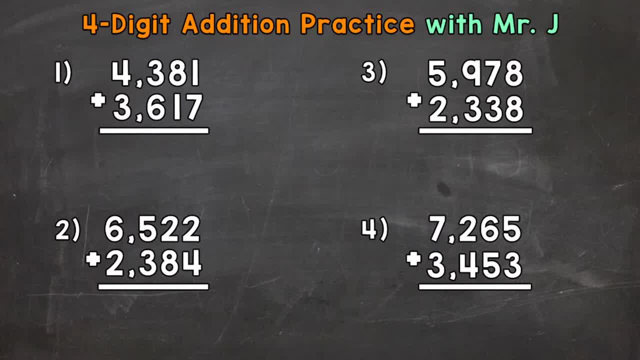 working with four-digit numbers. So let's jump into number one, where we have 4,381 plus 3,617.. Now, when we add whole numbers, we always start with the ones plus the ones that are in the middle. So let's start with the ones that are in the middle. 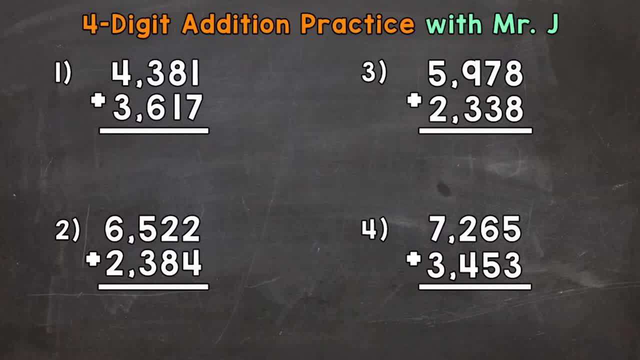 So we have 1,1 plus 7,1.. That gives us a total of 8,1.. So we have an 8 in the ones place. Then we work our way left to the tens place, So we have 8,10 plus 1,10.. That gives us a total of. 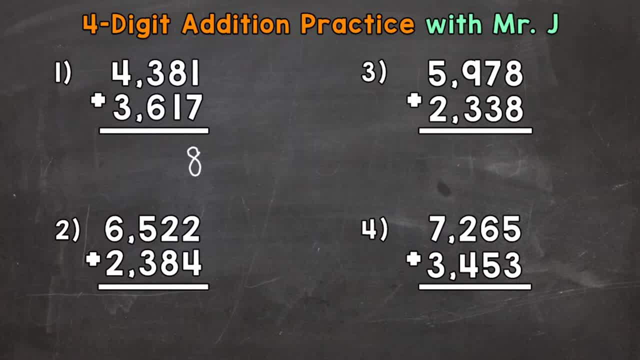 9,10.. 8 plus 1 is 9.. So a 9 in the tens place. Now we move to the hundreds place. So 300s plus 600s, 3 plus 6 gives us a total of 9.. So a 9 in the hundreds place. And lastly, 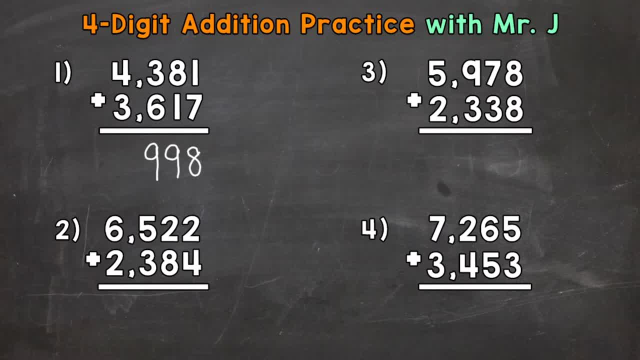 the thousands place. So 4,000s plus 3,000s, 4 plus 3 gives us a total of 7.. So a 7 in the thousands place, And then we put our comma in the answer And our final answer is 7,900.. 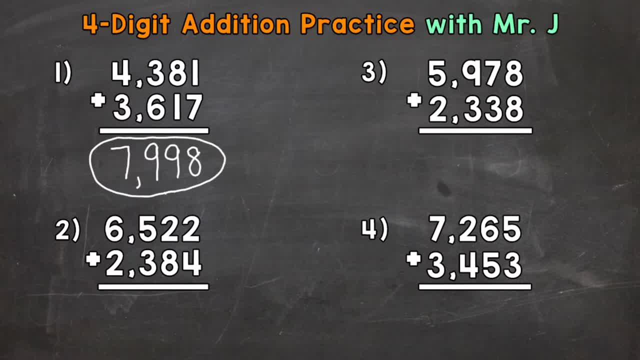 98.. Let's move to number two, where we have 6,522 plus 2,384.. Start with the ones. So 2 plus 4 gives us a total of 6.. Now for the tens. So 2 plus 8.. 2 plus 8 gives us 10. So. 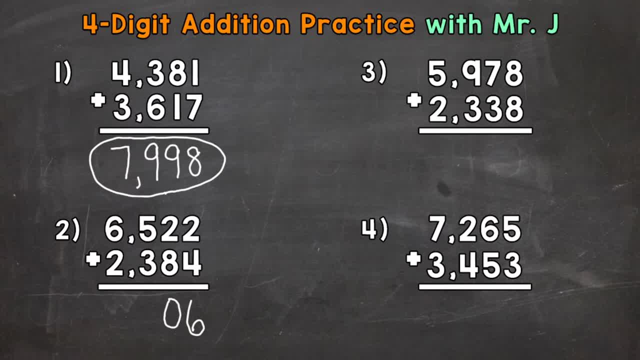 we put the zero from 10 in the tens place And then we have 8,1 plus 3,000s plus 3,000s. So we move to the hundreds place And we regroup the 1. So we have 8,, 4-. put todos in the. 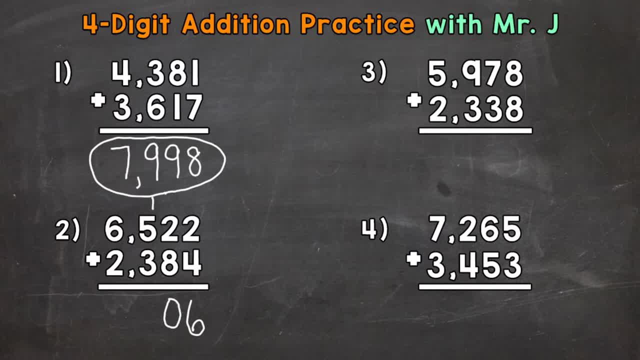 tens place And we regroup the 200s in the tens place And now we have 1 plus 5 plus 3 in the hundreds place. So 1 plus 5 is 6. Plus 3 is 9. So a 9 in the hundreds And. 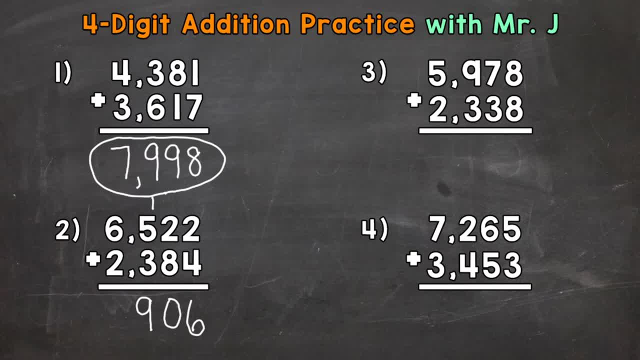 lastly, the thousands. place 6 plus 2 gives us an 8 in the thousands. Put the comma in our answer And our final answer is 8,000.. So 8 plus 6 in possono can give us slj workouto. Who knows where this list turned out in the. 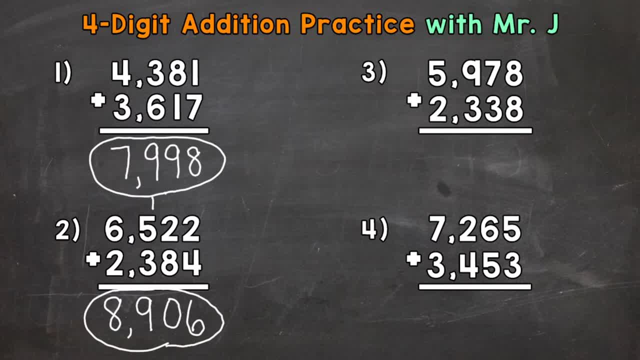 hundreds. place 6 plus 2 gives us 3.. 18 in the thousands place And finally, 3 to the thousands. pretend that you are advanced in math. That is BU Smith and re-group and change your reading. thousand nine hundred six. Let's move over to number three, where we have five thousand nine. 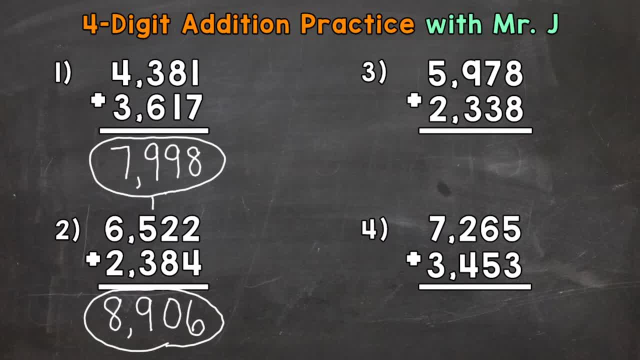 hundred seventy eight plus two thousand three hundred thirty eight Start with the ones. So eight plus eight gives us sixteen. Put the six from sixteen in the ones place and regroup the one over to the tens. Now we have one plus seven plus three in the tens place. So one plus seven is eight. 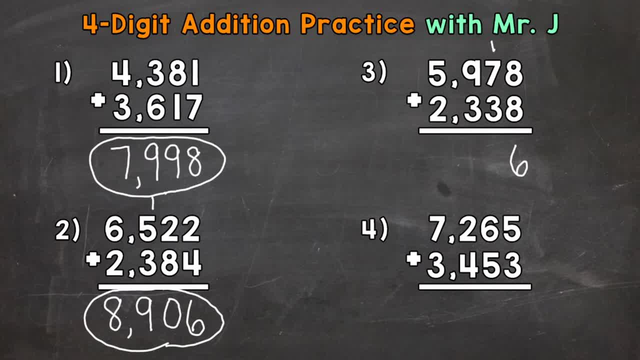 plus three is eleven. So put the one from eleven in the tens and then regroup the other one over to the hundreds. place Now in the hundreds. we have one plus nine plus three. So one plus nine is ten plus three is thirteen, So put the. 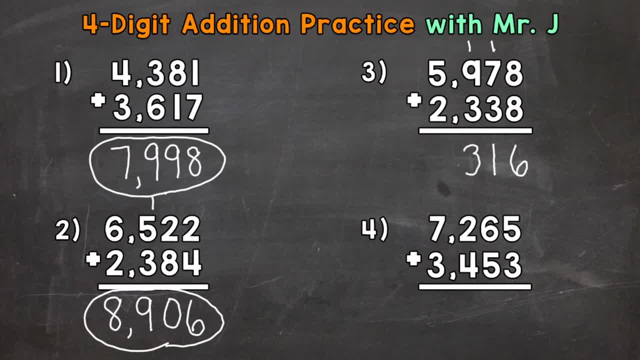 three in the tens place and regroup the other one over to the hundreds place. So one plus nine plus three from thirteen in the hundreds and regroup the one Now for the thousands. So we have one plus five plus two. One plus five is six plus two is eight. Put our comma in and our final. 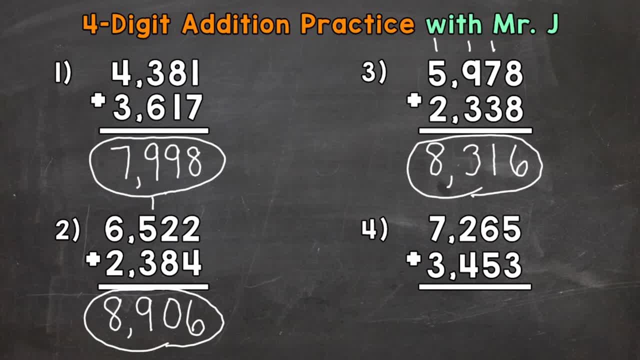 answer is eight thousand three hundred sixteen. Lastly, number four, we have seven thousand two hundred sixty-five plus three. So we have seven thousand two hundred sixty-five plus three thousand four hundred fifty-three. Start with the ones. Five plus three gives us eight. 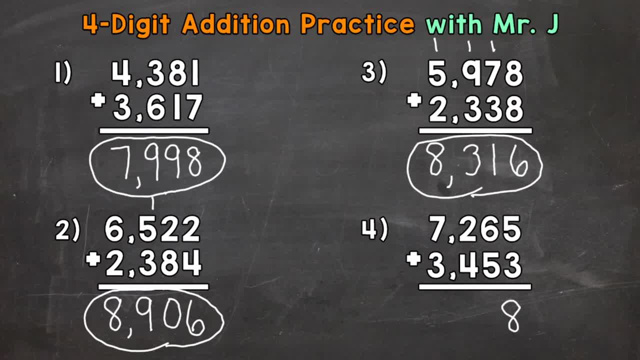 Now for the tens place. Six plus five is eleven. Regroup the one, Now we go to the hundreds. So one plus two plus four, One plus two is three plus four is seven. Now for the thousands, Where we have seven plus three. That gives us ten. So put the zero from ten in the thousands and